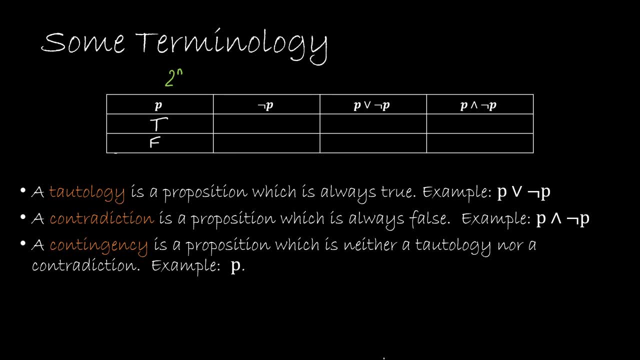 Not p is everything that happens in p negated, so true becomes false and false becomes true. Then remember, this is an or, so I'm looking at p or not p, and when we look at or, I want you to think about addition, because or is kind of like addition and in fact, in some 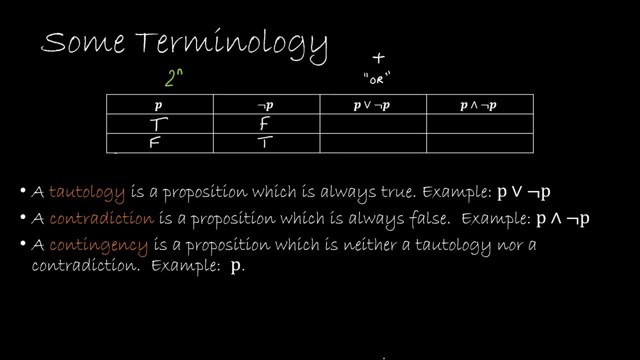 texts you will see: true displayed as 1, false displayed as 0. false is 0, true is 1.. And then if I'm taking, or what I'm saying is p plus not p, and p plus not p is 1, which is true, and 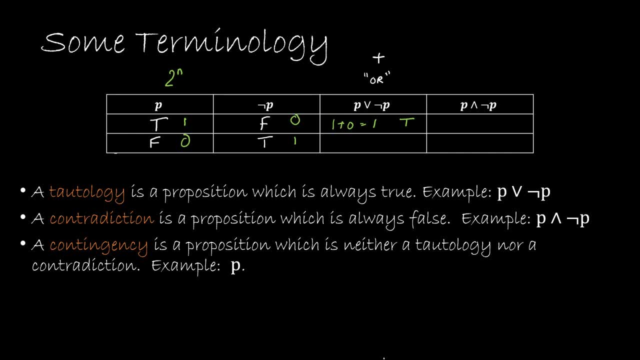 false, which is 0. P plus not P, which is true, equals 1 and 1, as we know is true. so what we call this is a tautology. a tautology is a proposition which is always true. so, as we can see, this would always. 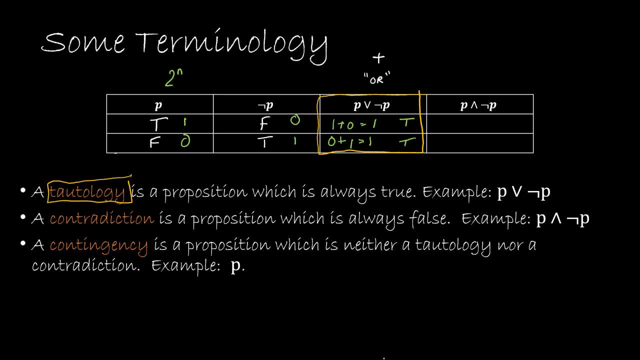 be true. so now think about it. if we weren't using ones and zeros, the way that we've talked about or before, is one or the other needs to be true for it to be true, and so obviously that's the case here and that's the case here. so whether we use plus or the reasoning that we used before, we still know. 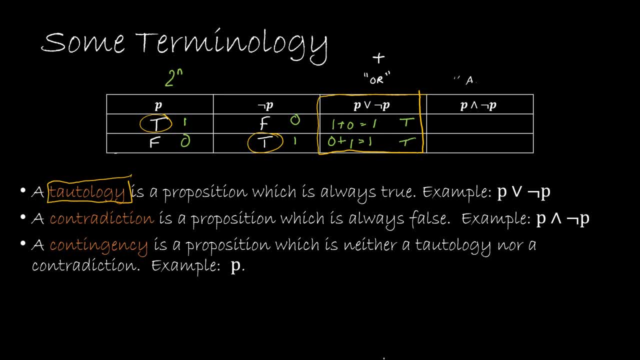 that's a tautology, this one is our, and, and I want you to think about that as multiplication. so I might think about 1 times 0 equals 0, or 0 times 1 equals 0, and either way I end up with false and again the way that we. 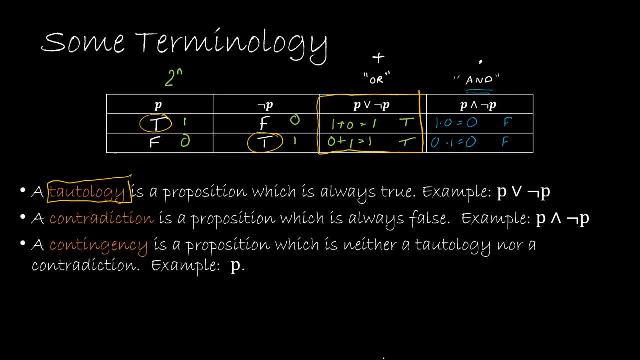 thought about it before. when we talked about and, and and was they both had to be true. and, as we can see here, they're not both true. and, as we can see here, they're not both true. this is called a contradiction, and a contradiction is a proposition which is always false. so here's my contradiction. 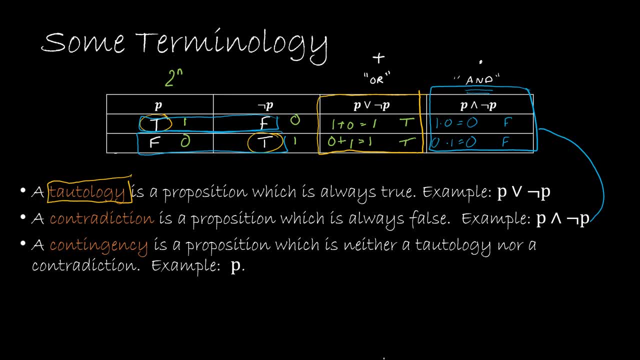 and here is my tautology. now, a contingency is a proposition which is neither of the two. so it's neither a contradiction or a tautology. for example, P. if we can look at the entries in my P column, I've got a true and a false, so it's not always true. it's not always false, it's a contingency. so we 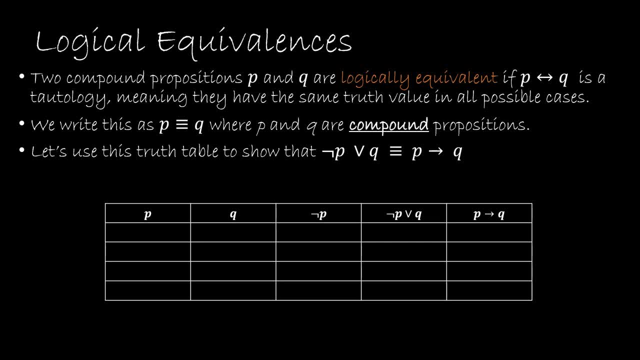 are trying to show you how to do this, so we're going to go ahead. and we're going to go ahead and show now that two compound propositions are logically equivalent. P and Q here are representing compound propositions, so I'm not using P to represent I went to the store and Q to represent 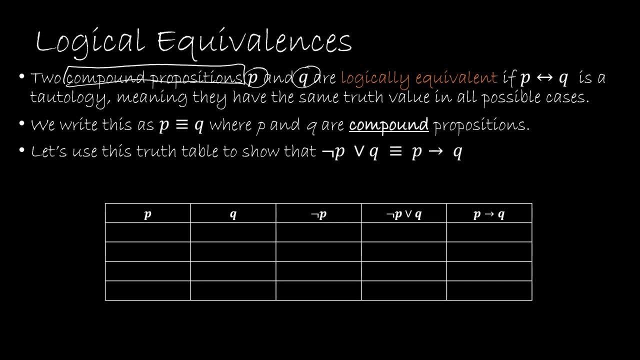 I bought a diet dr proper because they're delicious. I'm saying: these are compound propositions, so it could be something say like this or like this. so that's what we're going to do in this first example together. now to show the two compound propositions are logically equivalent. we have to show that P if 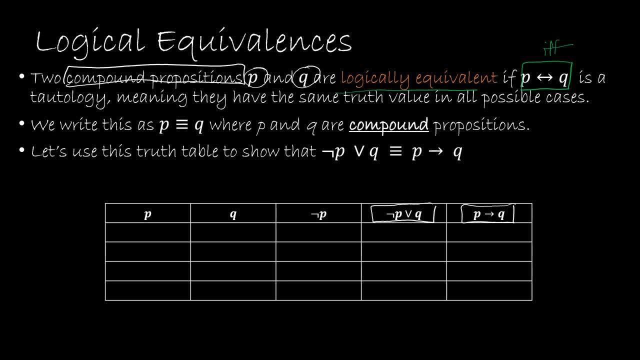 and only if Q is a tautology- remember, tautology tells us that it's always true- which means that those two compound propositions will have the same truth value in all possible cases. this is why a truth table is fantastic for this, because all I have to do is I'm going to go ahead and do. 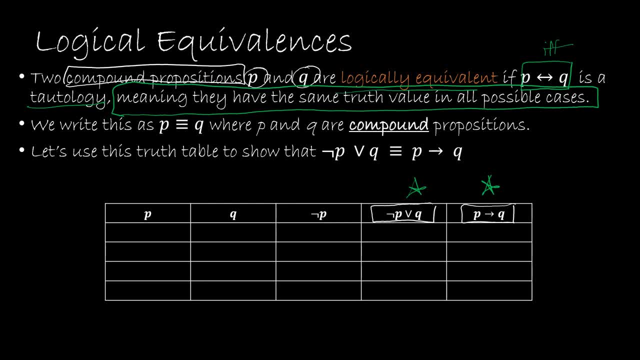 is create a truth table that gives me the truth values in all possible cases and show that they are equivalent. and again, we're going to use this sign to show that they are equivalent. it's kind of like an equal sign with an extra line and it means that they are logically equivalent. so let's try our. 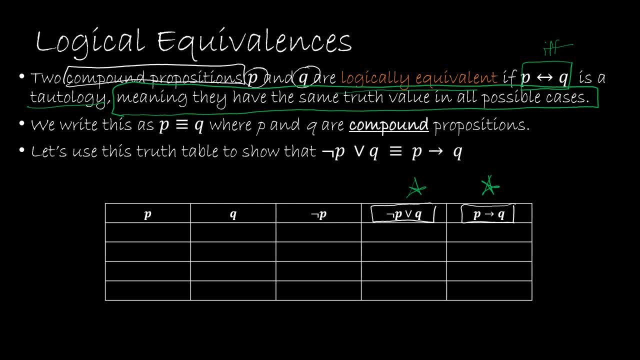 first practice question together, and just as a reminder, a truth table has three parts. on the left-hand side is all the way to the right, and on the left-hand side is all the way to the left, and on the right-hand side is always. however many propositions, we have all of their combinations. so 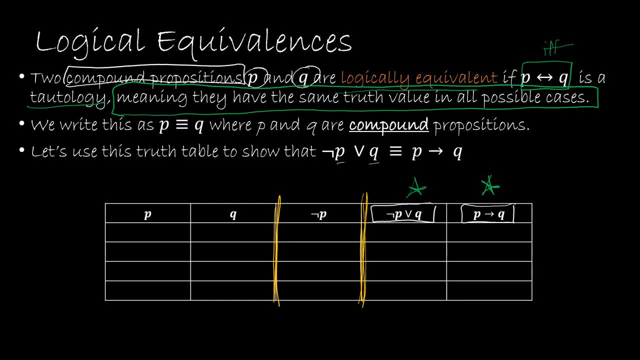 here, as we can see, I have P Q, so I have two of them. we take two to the however many propositions we have, and in this case, two, and that's where I got four rows. that's how I knew we needed four. then I start with true, true, true, false, false, true. 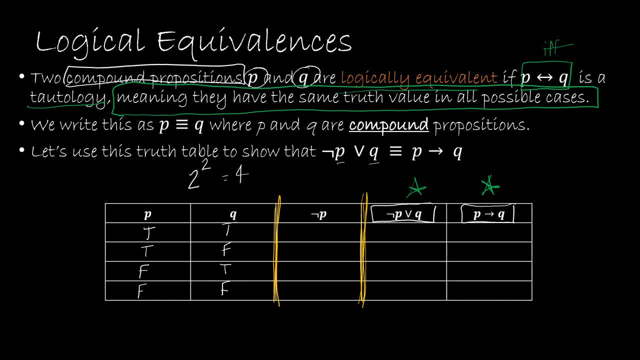 false, false. that's the first part of my truth table. the second part of my truth table- the middle- is always anything that I need, any parts that I need to get to my final conclusion. so sometimes you won't have anything there, but most likely you will. in this case, I just have one thing and that's. 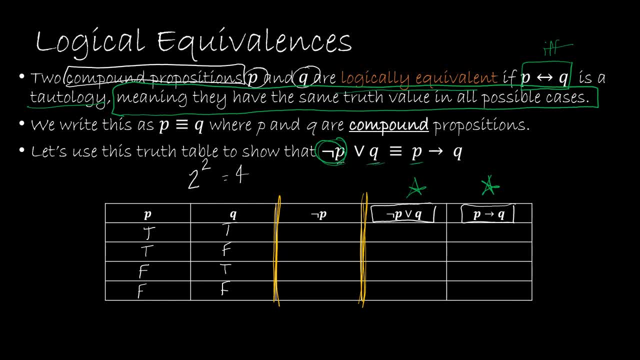 not P, because, as we can see, I already have a column for Q and for P and for Q, but I don't have a column for not P, so I need a column for that, not P. tells me that I'm taking whatever's in the P column and changing it, so true becomes. 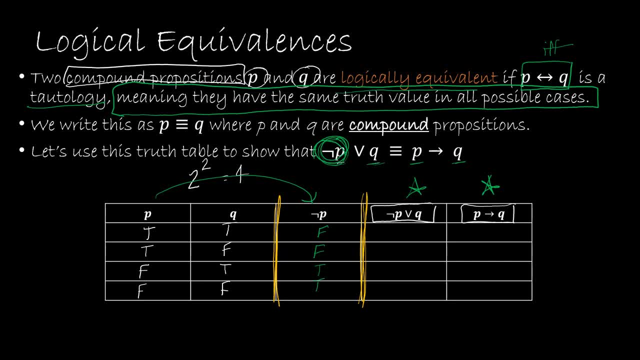 false. true becomes false. false becomes true, false becomes true. we negated it. that's the not P. I'm gonna try to get that T back in that box a little bit better. now we go to the third part, which is the important part. here, the important part shows us what is the truth value for, not P or Q. 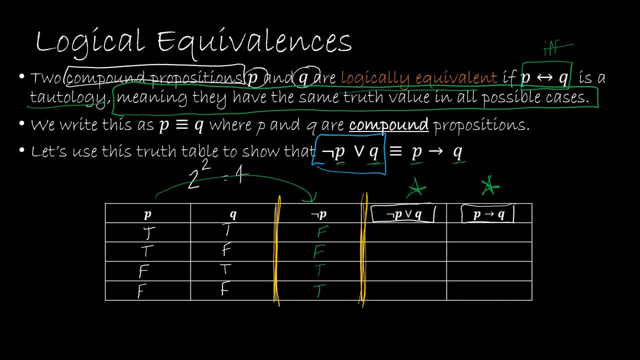 the important part shows us what is the truth: value for, not P or Q. so again, keep in mind this is an or, and when we're doing an or we're saying one or the other needs to have a true, so not P and Q. notice there's a true in what I just circled. this is a false, false. 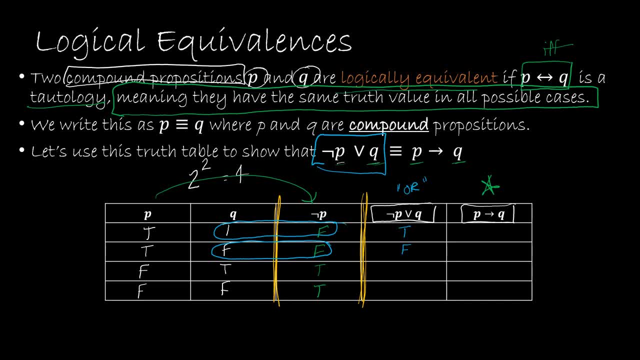 so there's no true, so the result is false. this is a true true. it's just fine to have two trues. and this is a false true, and I have at least one true, so it's true. now let's try my other compound proposition, which is: if P, then Q, which means 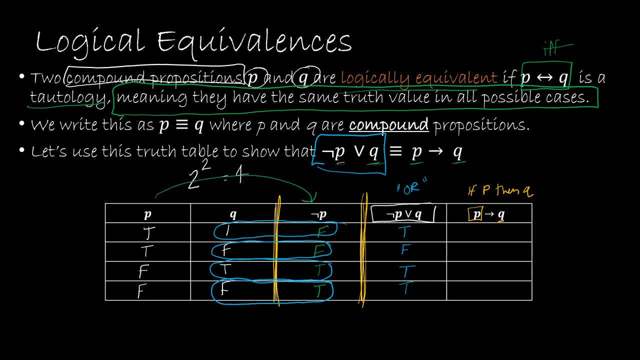 if P is true, then Q must be true to return a true value. and if P is false, then it's true. so here I have true, true. well, if P is true, Q must be true, and that is the case. here I have true, false. so here I have true, true. well, if P is true, Q must be true, and that's not the case, so it's false. 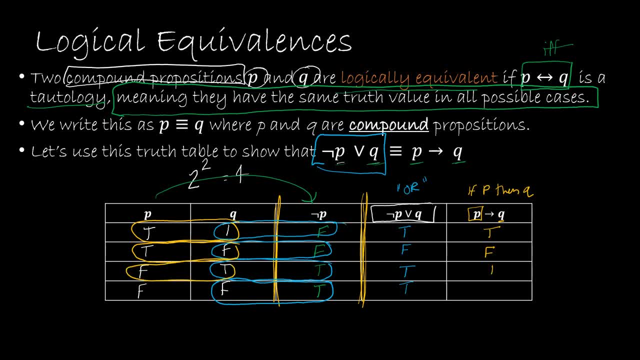 if P is false, it doesn't matter what Q is. the result is true. so here's my result. then we examine the two and typically I just put a box around them and say, hey look, yay, these two match up. therefore, I have demonstrated that the two compound propositions. 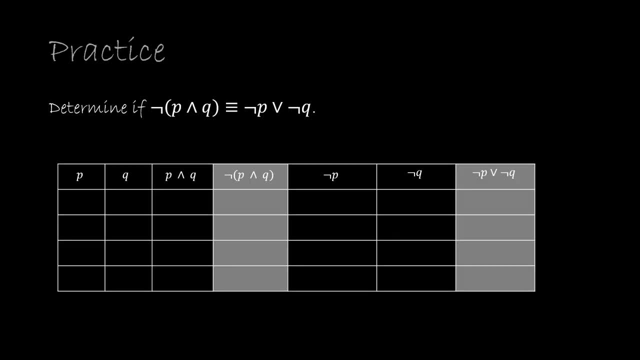 are logically equivalent. here's one more practice for us to try together, and again, I've cheated a little bit and already set this up for you, but it's important that you know how to set it up yourself. so if you don't, I'm going to go through that very quickly. if you already know what you're doing, you can go ahead. 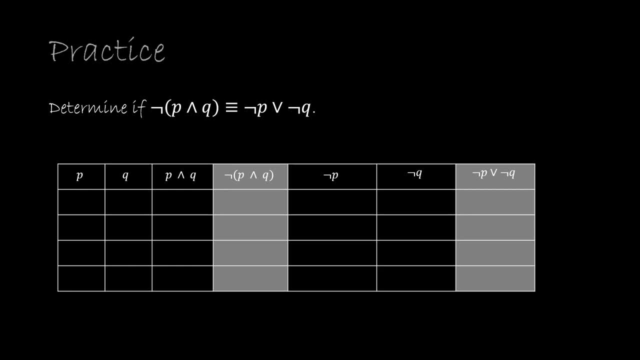 and start on the truth table and just ignore me talking to you. so again, what I would do to start is say: how many propositions do I have? I have P and Q. that's two. so I take two to the second power because there's two propositions. so that means I need four rows. 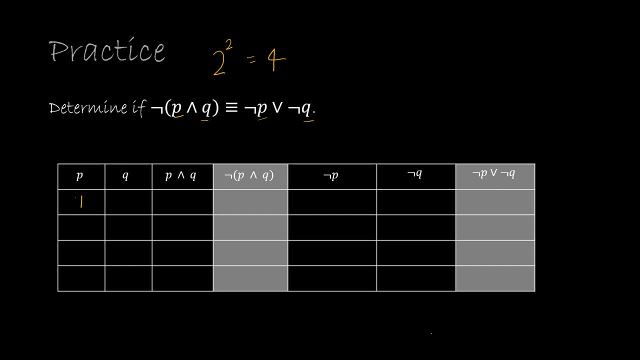 I need a column for P and a column for Q, and I can go ahead and fill in: true, true, true, false, false, true, false, false. yes, I'm going through that part kind of quickly. then I need a column for every part of a proposition, so I have P and Q here, and then my final solution is not P and Q, and then I've got. 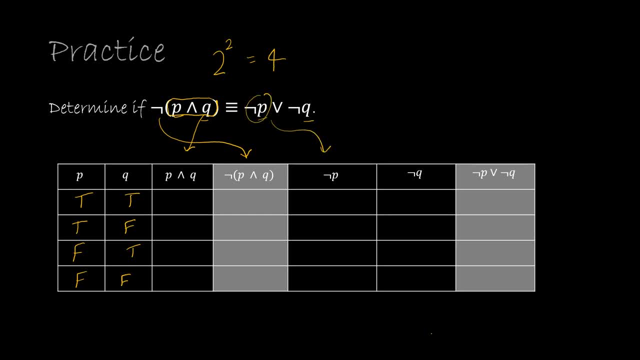 not P, which I need a column for, and I've got not Q, which I need a column for, and then I've got my final result, which is not P or not Q. so now that I have everything set up correctly, let's go ahead and work on this, my first column that I'm going to fill in. I'm going to get rid of all of these. 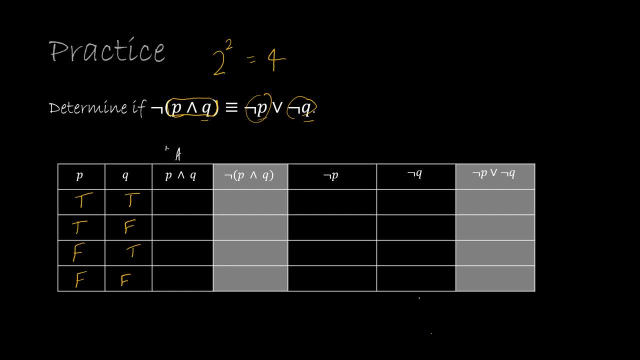 pesky arrows is P and Q, and remember for an and both values must be true to result in a true. so P and Q, which is true, true gives me a true. this one they're, but not both true. they're not both true here. they're not both true here. so there's my new column now to fill in. 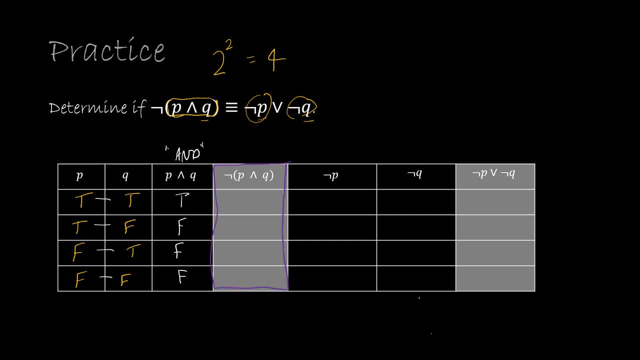 not P and Q negates anything here. so true becomes false, false becomes true, false becomes true, false becomes true. So that is the column that I am going to compare over here. So let's go ahead and fill in what we need to for the other columns. 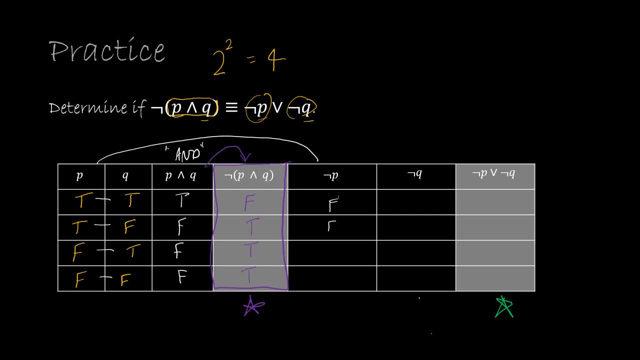 This is not P, so that becomes false, false, true, true. This is not Q, which becomes false, true, false, true. And then this one is not P or not Q. So remember, when you're dealing with an or you're dealing with one or the other must be true. 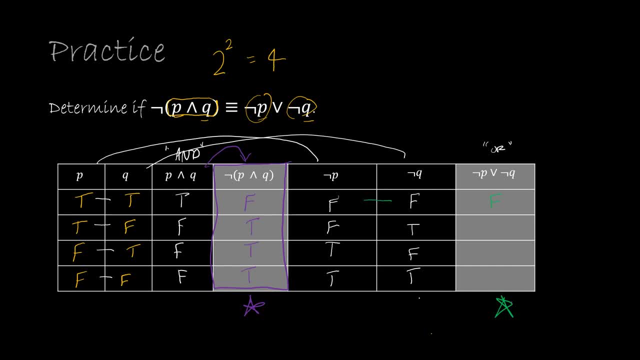 So is one or the other true? No, so it's false. Is one or the other true? Yes, yes and yes. Sorry, you can't see that very well. False, true, true, true. So, as we can see, comparing this column with this column, 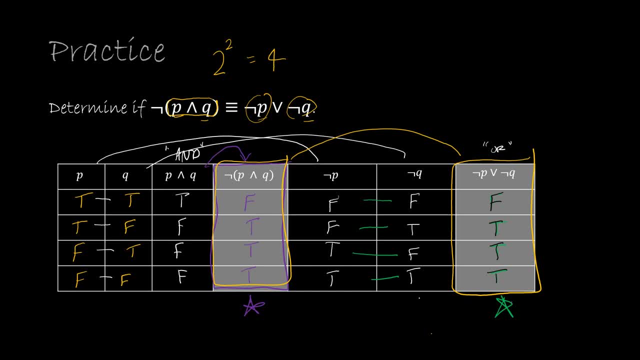 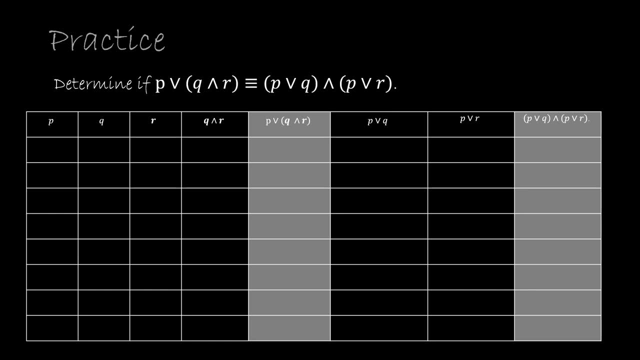 we see that they are logically equivalent because they return the exact same truth values. Here's one for you to try on your own. So, if you would press pause, try this question and then, when you are ready, press play to see how you did. 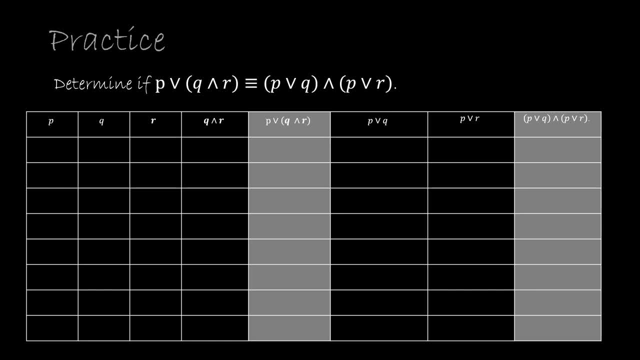 So the part that hopefully should come pretty quickly for you and, again, hopefully you understand how to actually set up this table. But remember, here we're just going to do true, true, true, true, False, false, false, And then true, true, false, false. 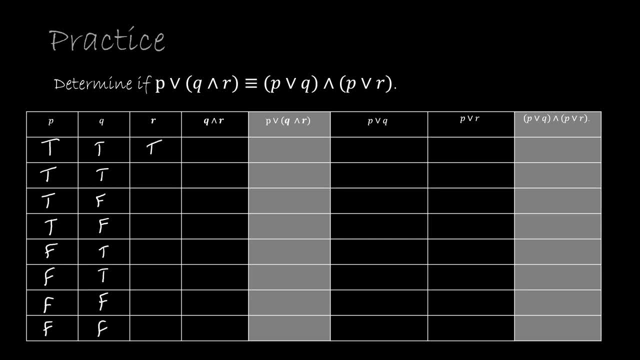 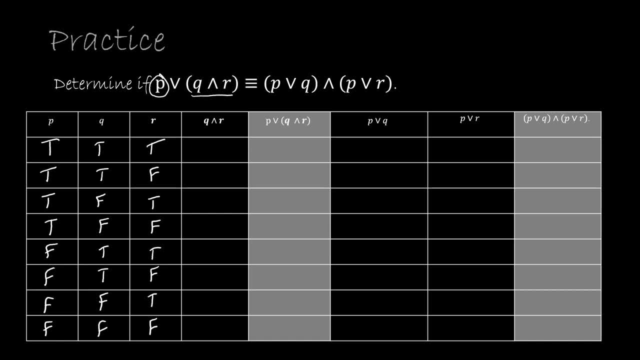 I needed to create a column for Q & R. I needed to create a column for P or Q and create a column for P- I'm sorry- P or R, and then, of course, the ones that I have in gray are the complete compound proposition that we're going to be comparing. So, without further, 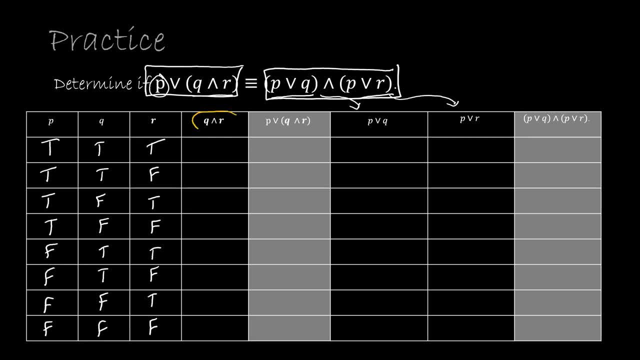 ado, let's get started Here. we have Q and R, and remember that means both of them must be true for this to be true. So that's a true, that's a false, that's a false, that's a false, that's a true. 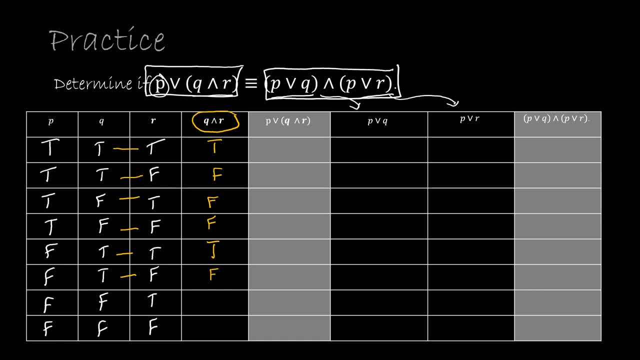 since they're both true. Since we have a false there, we have a false. Since there's a false, we have a false, and then two falses make it a false. So far, so good. Now let's go ahead and find this column. I'm just going to use black here. so we're going to say this is: 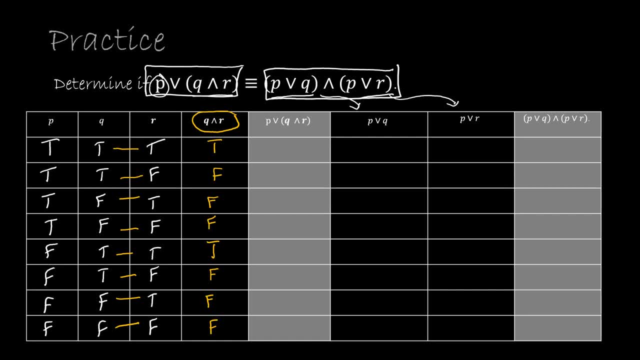 P or Q and R. So I'm looking at: let's use green, this and this. So these are the ones that I'm looking at and remember, if it's an or we're saying one or the other must be true, and if one or the 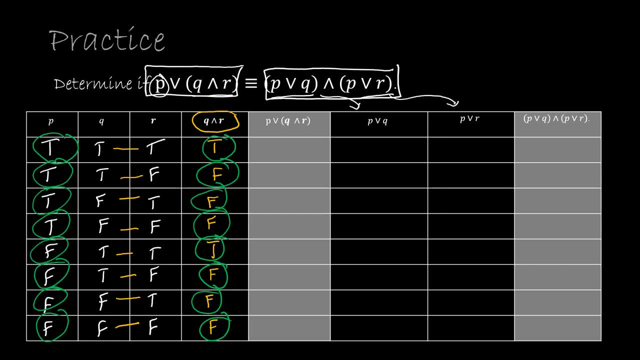 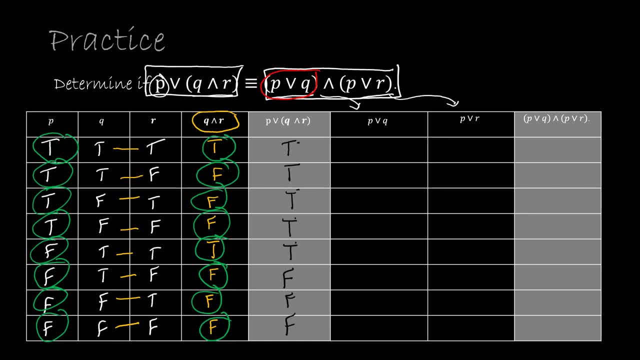 remember that's an or so. that means either one can be true. So I'm looking at true, True, True, True, And again I'm saying true every time there's a true in what I'm circling: True, True, False And false. Now I'm going to do the same, but